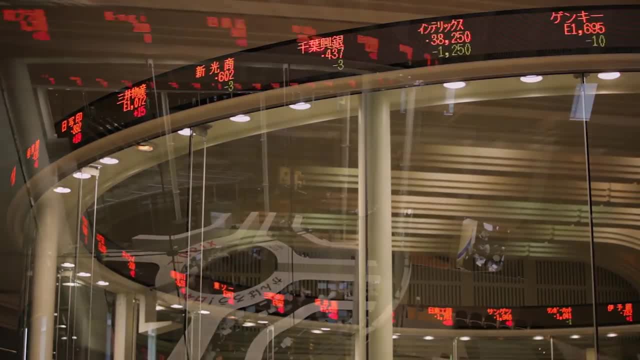 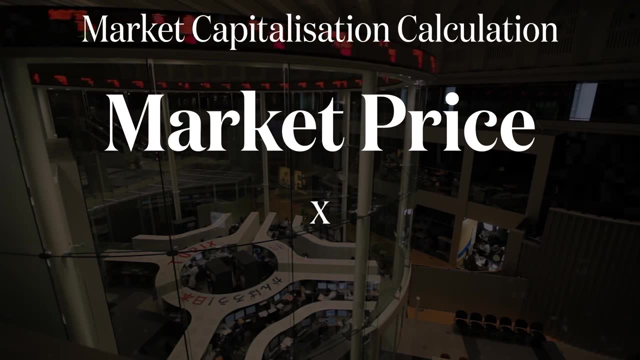 So the first thing to know here is that market capitalizations are sometimes a bit misleading. This number is calculated by taking the market price of a stock and then multiply it by the total number of stocks. there are currently just under 1 billion Tesla shares in existence. 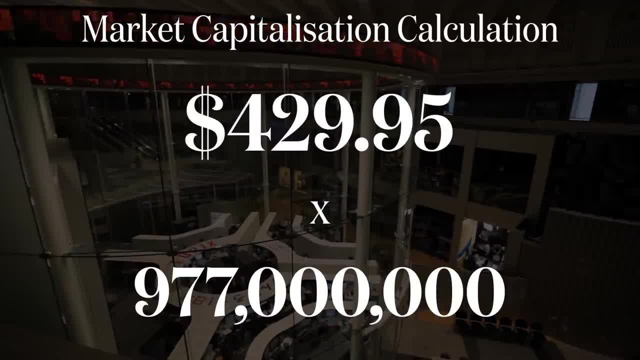 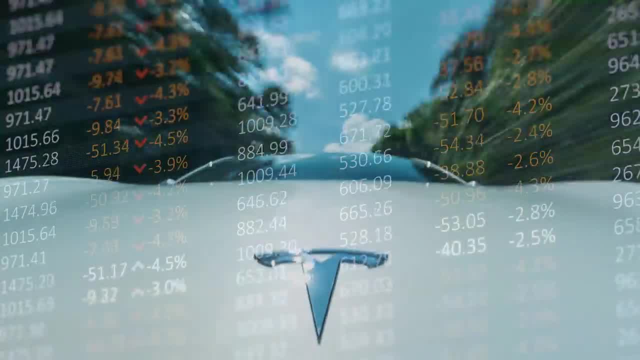 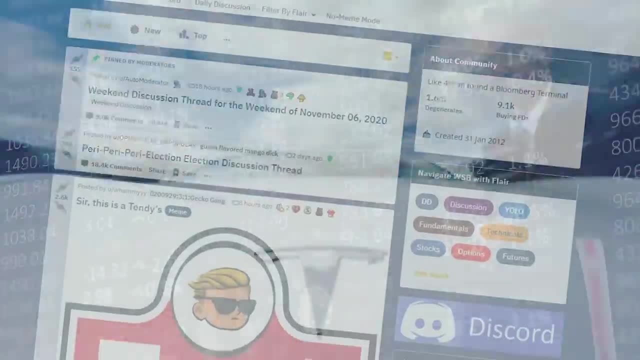 so if we multiply that by the 430 dollar market price, we get ourselves a market capitalization figure. So now the market price is something that can jump around quite a lot for any number of reasons that are completely divorced from the underlying fundamentals of the company: amateur investors, stock buybacks, easy access to capital. 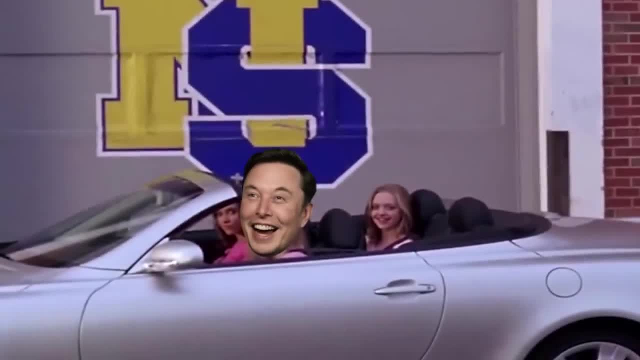 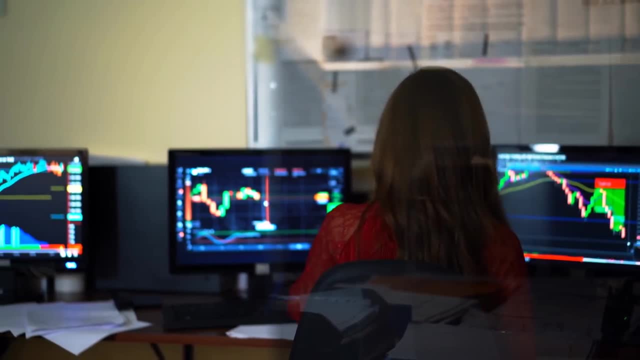 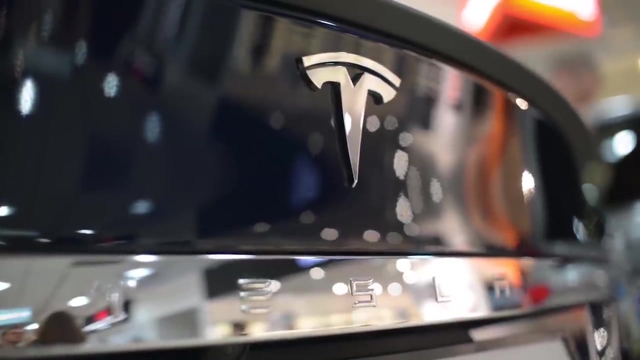 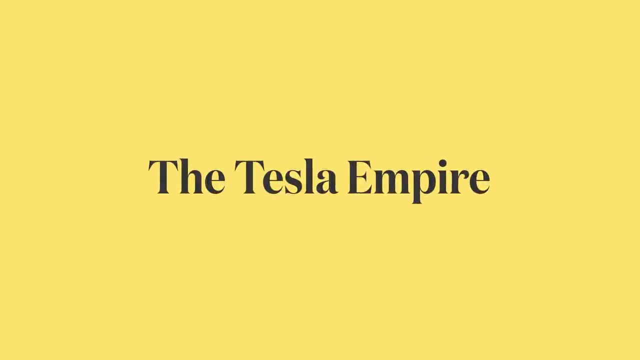 price Money, manipulating tweets- all that good stuff can push the share price up or down without actually making the company they reflect any larger or smaller or more prosperous. All of these factors are common criticisms levelled at tesla, but supporters will point to the fact that building cars is just one small part of scaling up the tesla empire. 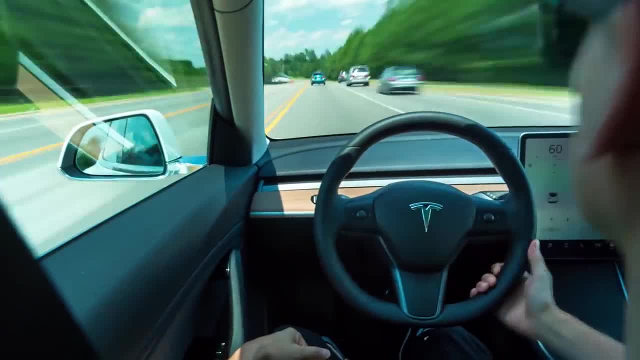 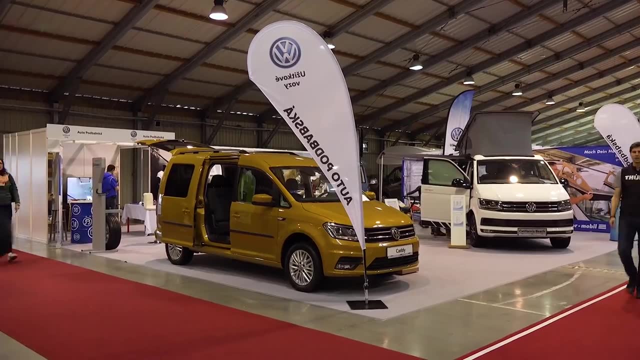 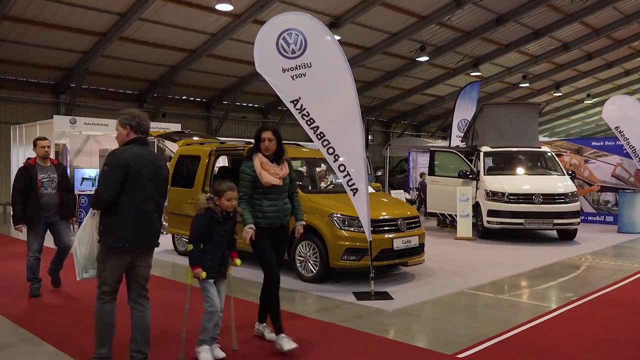 One of the most telling insights into the difference between tesla and regular automakers is to look at their subsidiaries. Regular automakers have grown their influence by buying up other car brands. Volkswagen is a great example of this. Volkswagen group is not only responsible for the people's car, but they also own a part. 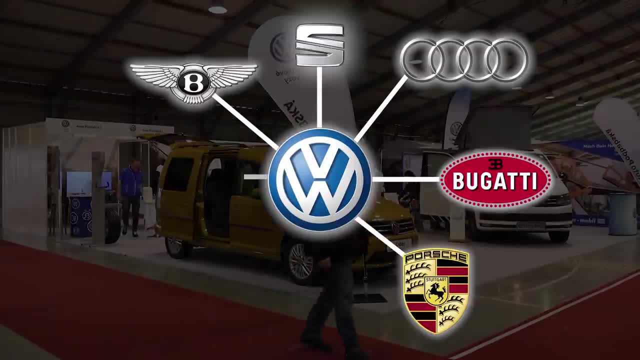 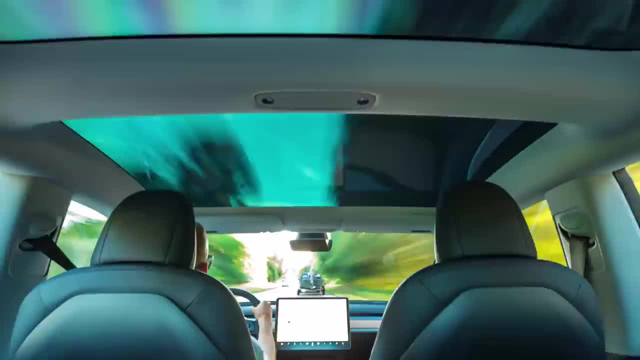 or all of Bentley, Audi, Bugatti, Porsche, Seat, Lamborghini, Skoda, as well as a collection of commercial vehicle manufacturers. Tesla, by contrast, is a company that still owns other companies, but it takes a slightly different approach to its mergers and acquisitions. 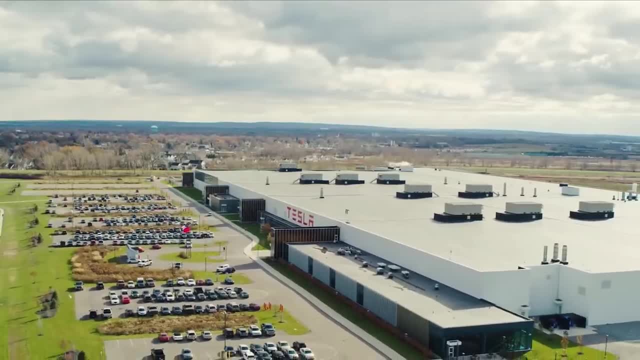 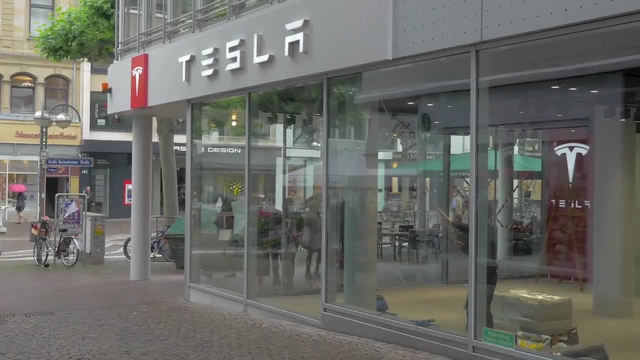 Instead of buying up competitors, it owns companies within its own supply chain, which allows it to not only be a car manufacturer, but also a component supplier, a dealership, a fuel station, energy generator and, maybe even, one day, a transport provider. all of its 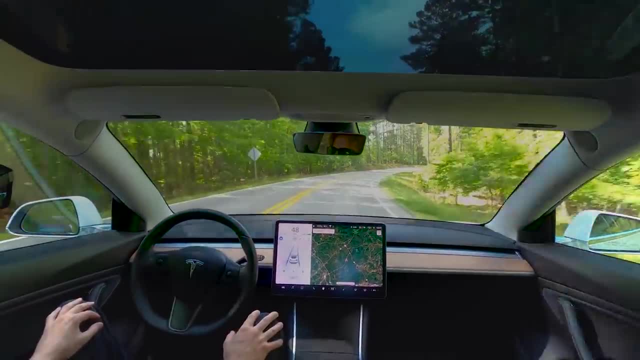 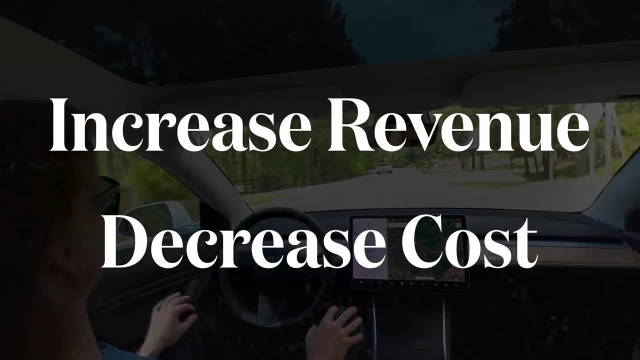 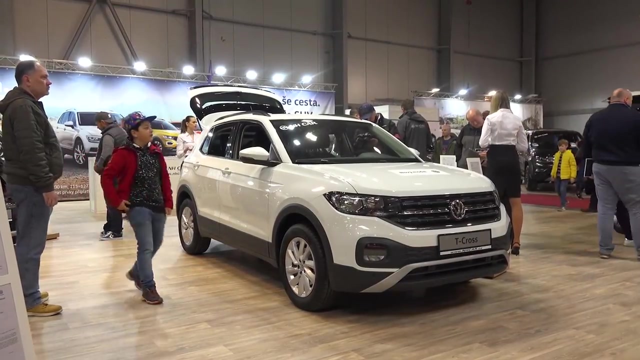 own. Now. these two different approaches all hope to achieve the same two things: increase revenue and decrease costs, which results in increased profits. Business 101 right, But here is how they do it. A company like Volkswagen is investing in what is known as a horizontal integration. 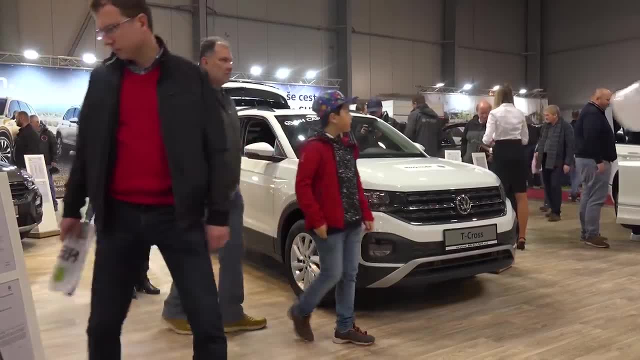 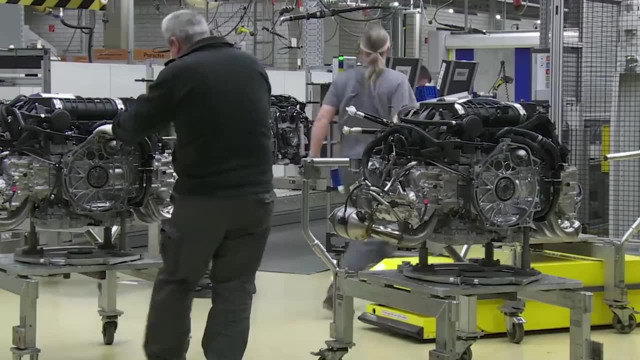 ie they are investing in businesses on the same level of the production process as their own. Porsche and Volkswagen are companies that technically do the same thing. They take raw materials and component parts and turn them into cars before selling them off to dealership networks. 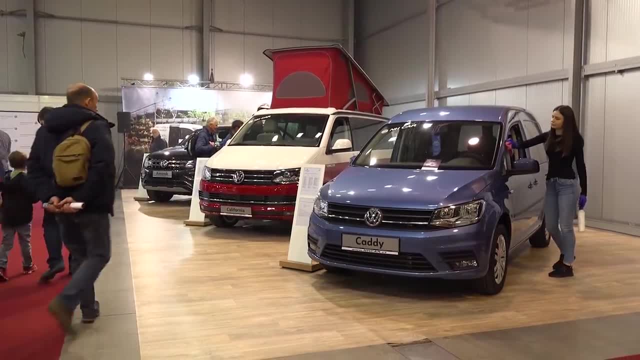 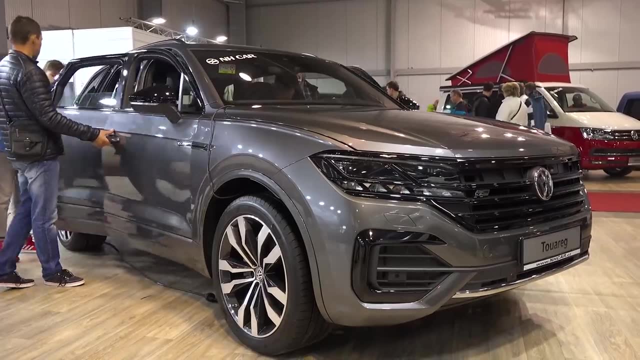 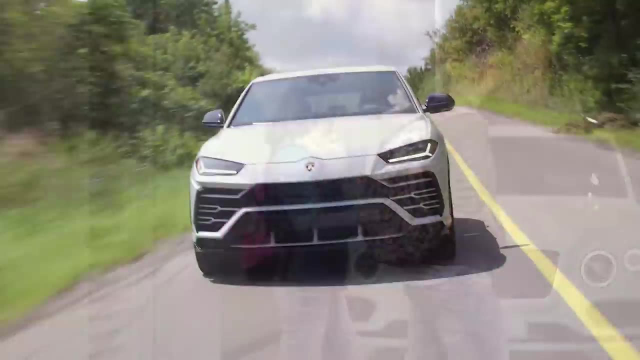 Now, just because all of these car companies do the same thing doesn't mean that there aren't huge advantages to teaming up. Companies like Volkswagen Will build cars on similar platforms and share them between all their brands: The Volkswagen Tiguan, Audi, Q7,, Porsche Cayenne, Bentley, Bentayga and even the Lamborghini. 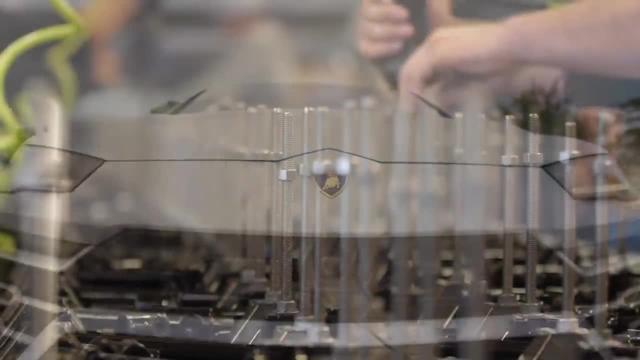 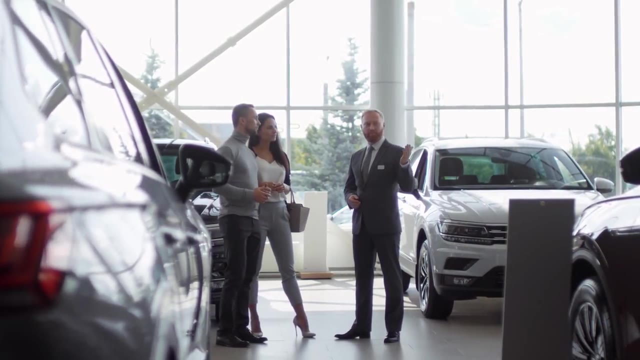 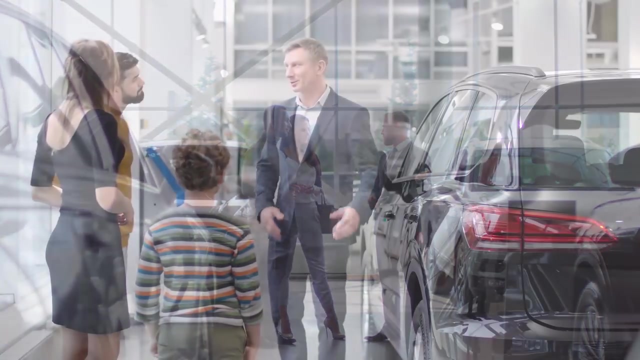 Urus all share the same components and chassis. This achieves the two things the business wanted to do. It increases revenue because suddenly the manufacturer can appeal to all manner of different buyers with effectively the same car. An average family gets a base model Volwtwagen. a wealthier family will buy a Porsche or Audi. 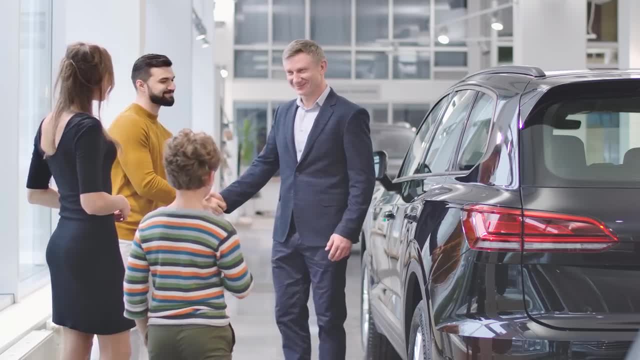 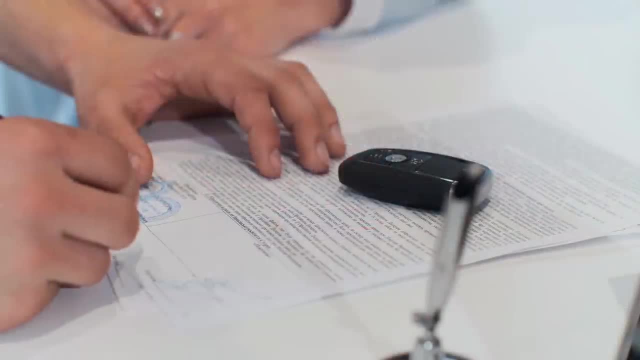 and for the people that buy cars- they could use their cars as well- want a truly ostentatious display of wealth. there are the Bentleys and Lamborghinis that cost six times as much for effectively the same car. This means that Volkswagen will draw revenue from buyers that don't want to consider. 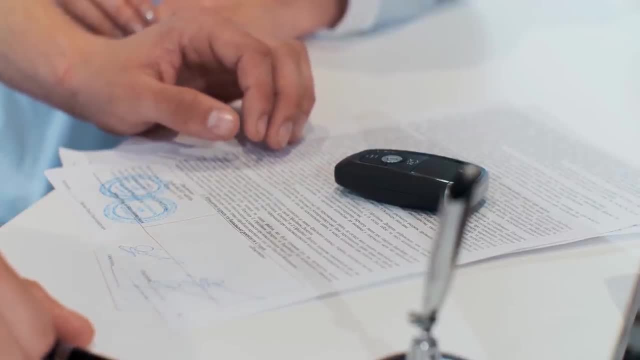 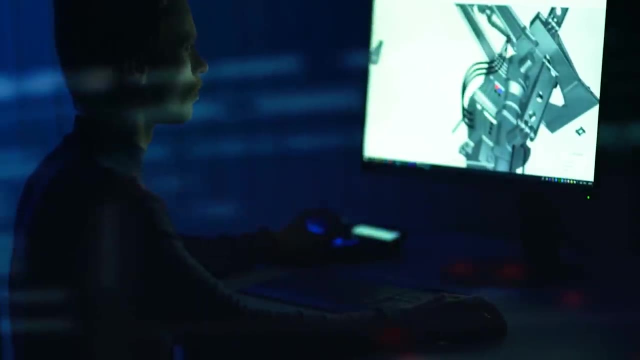 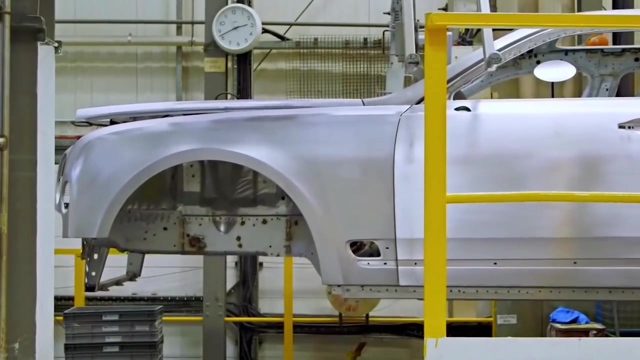 a car from the other end of the spectrum, either because it's far too expensive or far too povo. This technique of shared platforms also reduces costs because research and development, as well as manufacturing overheads, are shared between all of the brands. It would be cost prohibitive for a boutique manufacturer like Bentley to invest the same. 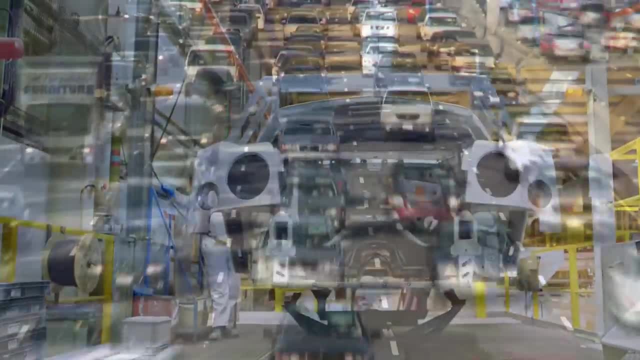 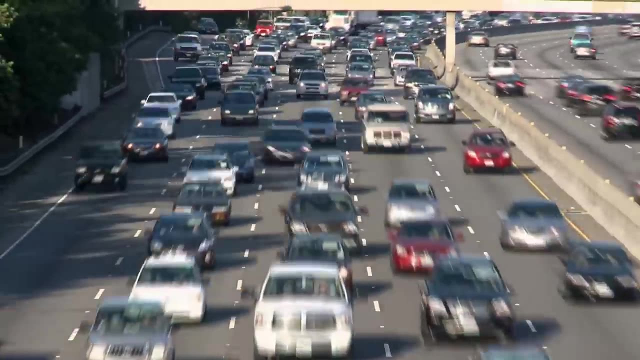 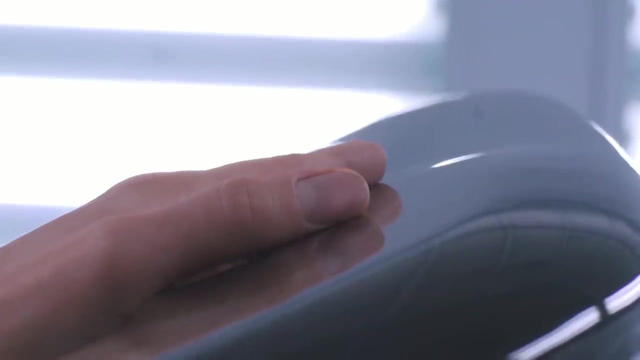 amount of money into developing a new drivetrain. Modern cars require huge teams of engineers, designers and lawyers to make sure that cars comply with all of the various road laws around the world, while also being a good car. And yes, yes, I know there are boutique manufacturers out there that do pull this off without being 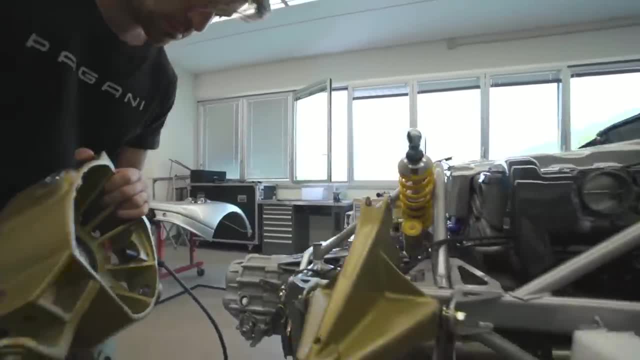 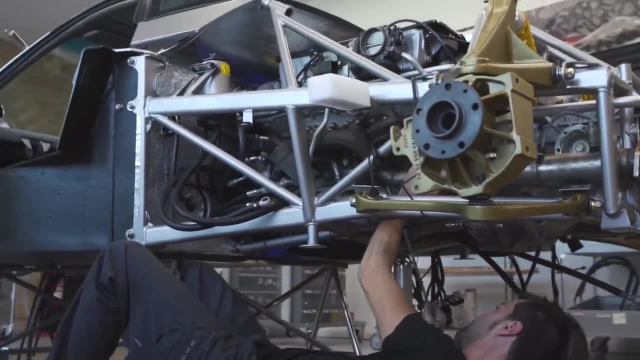 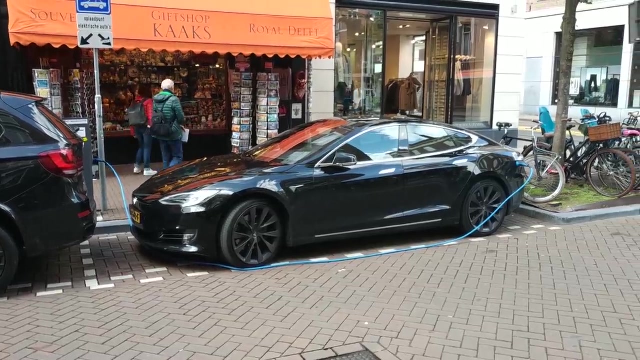 beholden to some corporate overlord. but just remember, those cars tend to be extremely expensive in the first place. They even buy Bentley and Lamborghini standards and they probably lack the day to day reliability as well. Tesla takes this expansion concept and turns it on its head literally. 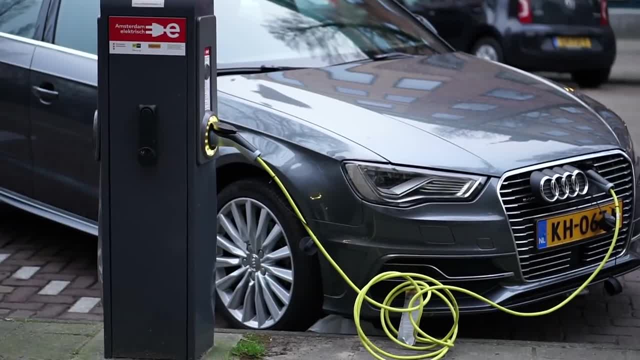 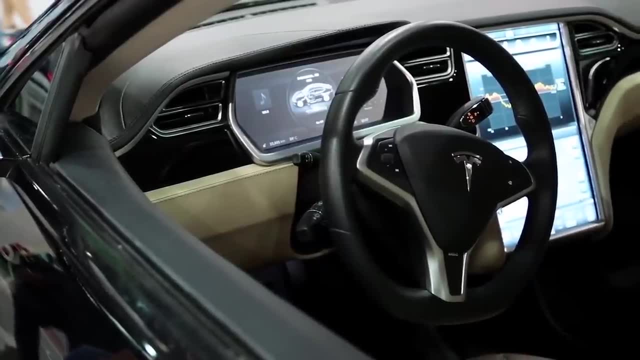 It does what is called vertical integration, where, instead of buying up competitors in the same step of the production process, it buys up or creates businesses that cover other parts of the process. Tesla's largest investment has not been into the cars themselves, but rather into component 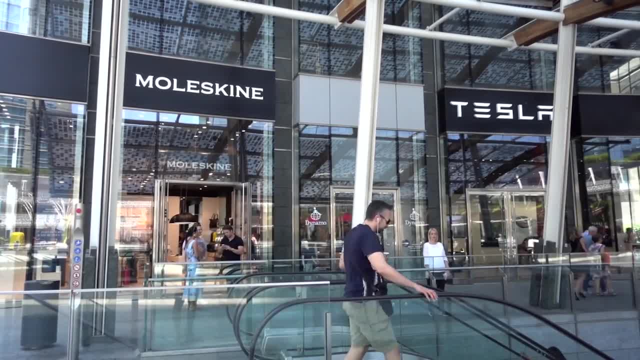 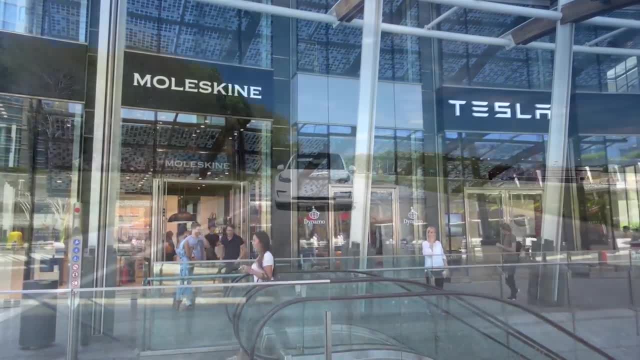 manufacturing recharging stations and owning their own dealership networks- all steps in the process of selling a car that traditional manufacturers have left to other companies. This achieves the same two goals: It reduces expenses because you don't have to include profit markups for all of the different. 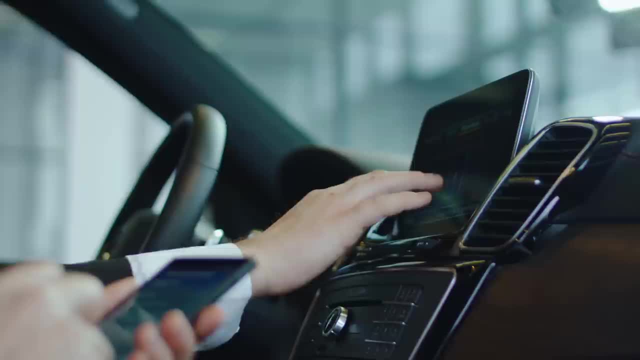 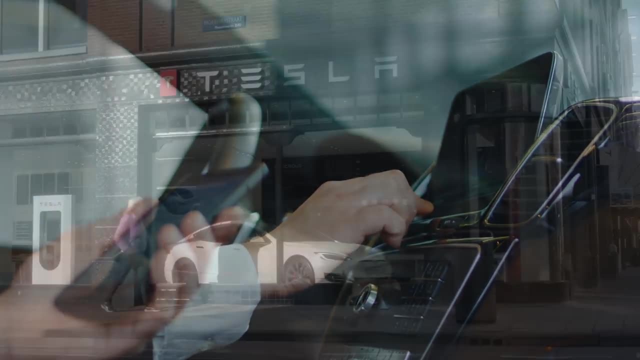 steps of the process. For example, if Audi sells a car to a dealership, they are going to sell it at a wholesale price, and then that dealer will add a markup to the consumer to make their own profits. By owning this entire process, Tesla can cut out those minutes. 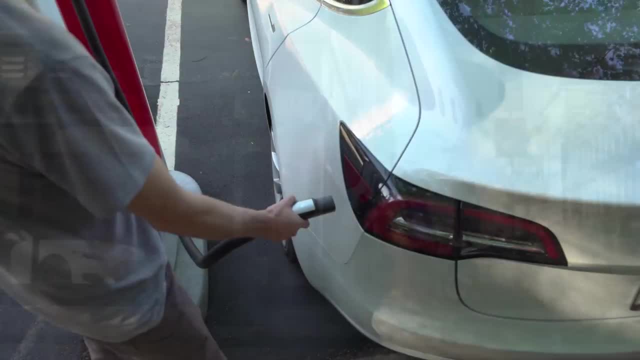 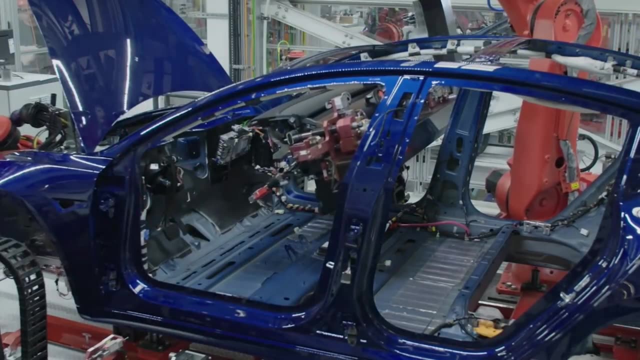 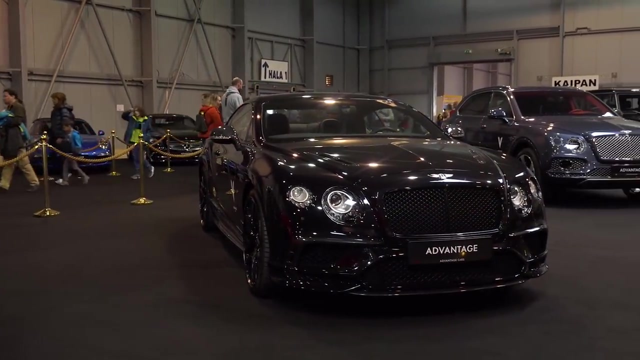 Tesla can cut out those minutes. It also increases revenue by offering additional revenue sources. Tesla really only makes three cars at the moment: the model s, the model 3, and the model x. We have just seen that the Volkswagen group has a wider selection of products within just. 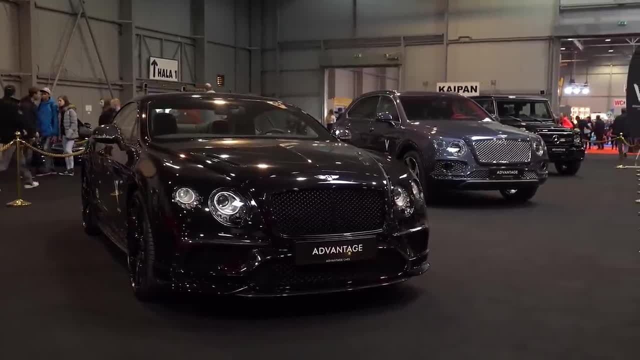 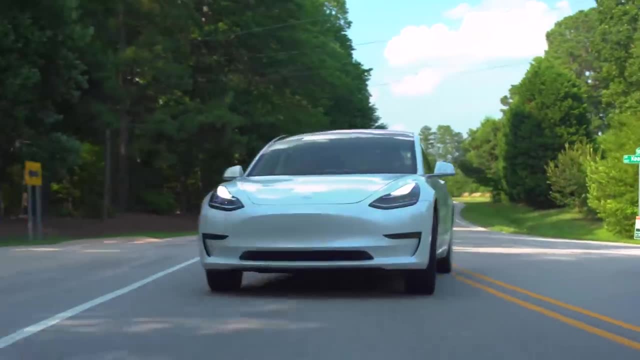 one chassis. But in the same way that Volkswagen increased revenue by offering lots of different types of cars to lots of different types of people, Tesla is offering lots of different services to the same types of people. If you buy a new Porsche and then go fill it up down the road, Volkswagen is not seeing. 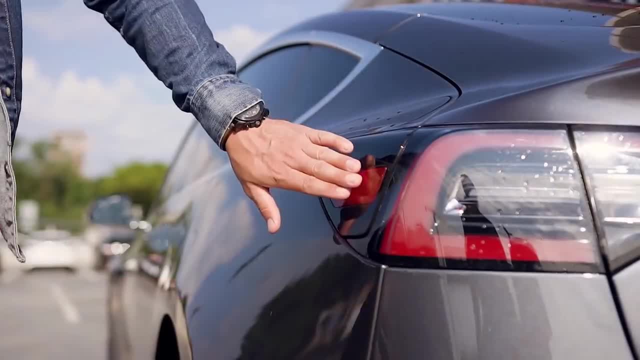 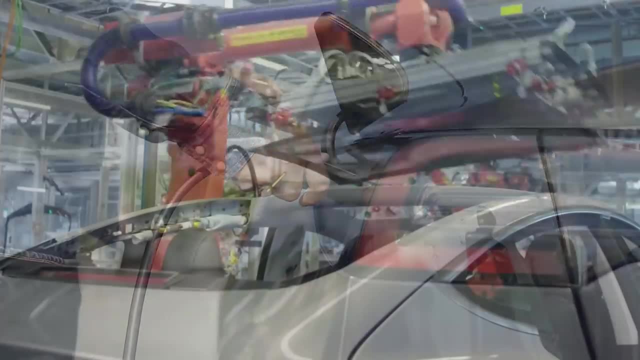 any revenue from the sale of that gasoline, Whereas if you buy a new Tesla and go charge it at the company s supercharger network, they will. The same is true for a lot of other areas as well. A byproduct of making electric cars with an emphasis on vertical integration is that 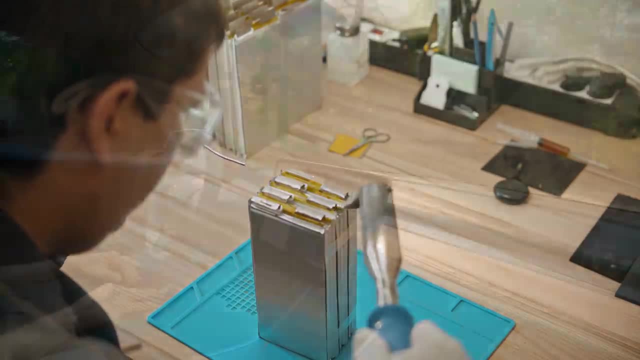 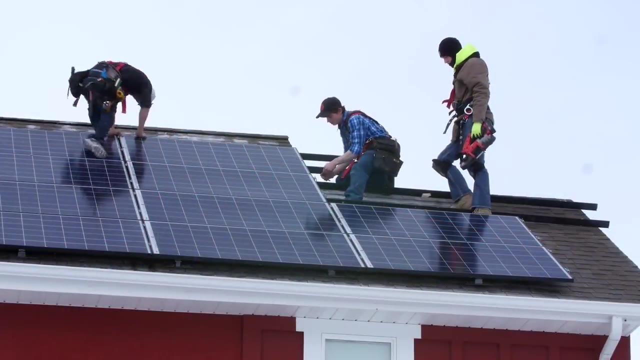 Tesla has become really good at making batteries. The same tree-hugging tech bro that will inevitably buy a Tesla may very well buy a house with a battery pack as well, Meaning that again, they have made money outside of just being one of the many moving. 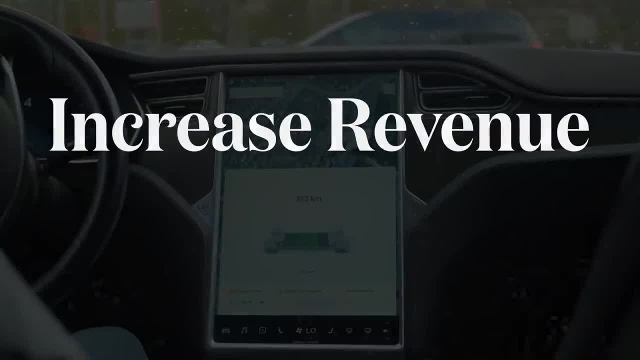 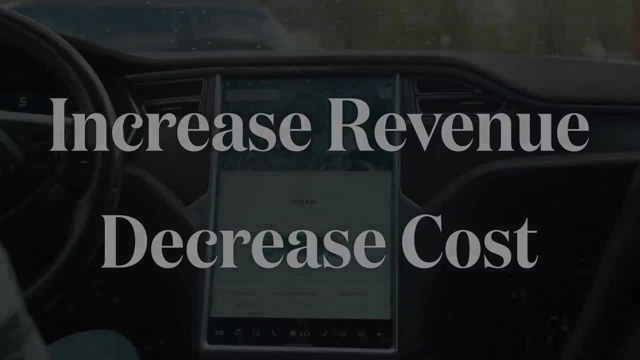 parts in the auto industry. So increase revenue and decrease costs to make more profit. Simple formula with two very different approaches from established automakers and Tesla respectively. The only problem is that, as innovative as Tesla s fresh new approach may seem, it hasn't. 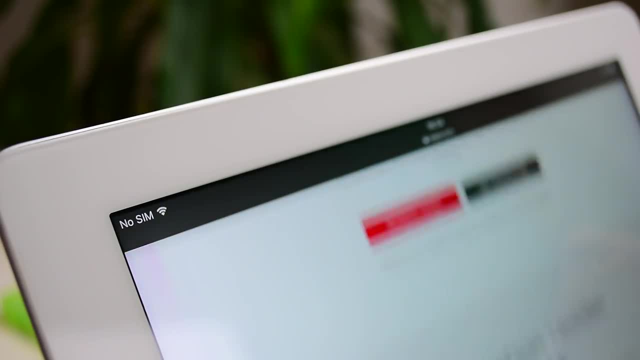 really worked. They haven't made any profit. To the contrary, they are losing money, But maybe that's okay Because they haven't yet achieved what they want to achieve. They are losing money, But maybe that's okay Because they haven't yet achieved what they want to achieve. 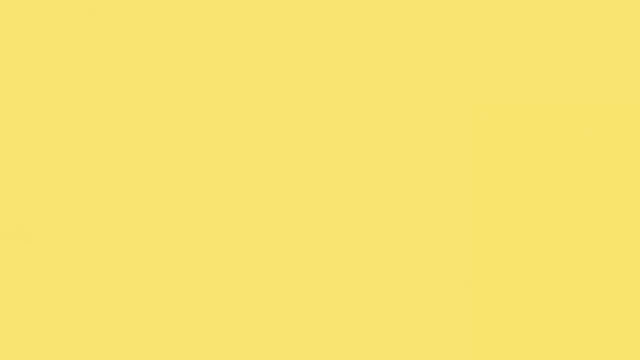 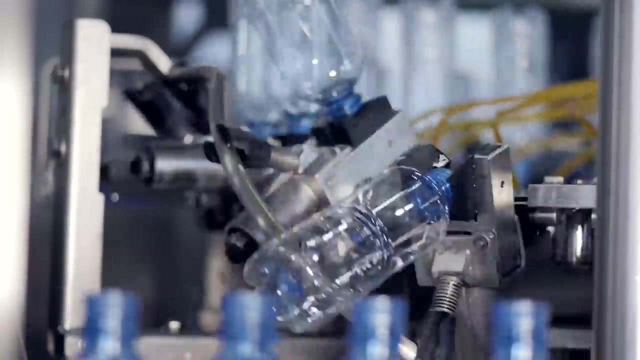 They are losing money, But maybe that's okay Because they haven't yet achieved what they want to achieve. The magic solution to all business woes: Economies of scale. Economies of scale is a phenomenon in production where the unit cost of goods trends downwards. 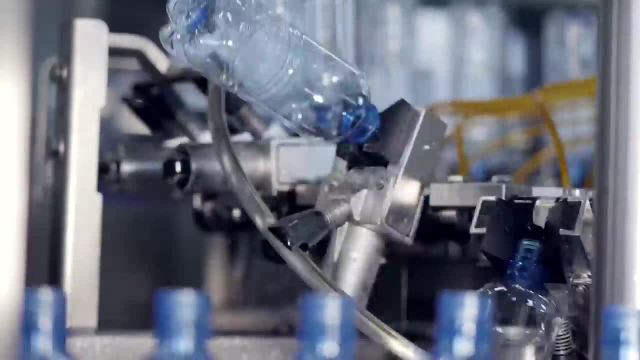 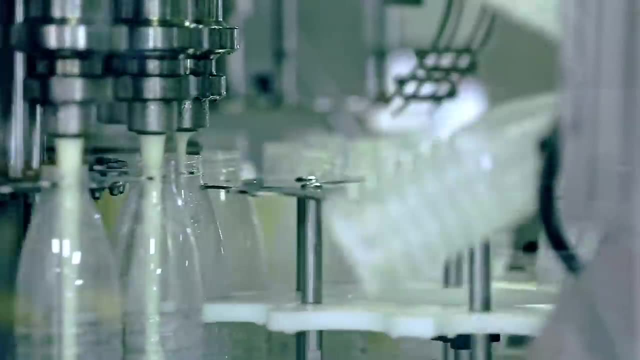 as more items are made. This phrase tends to get thrown around pretty loosely, but it's actually a lot more complex than what most people think. There are three main reasons why this happens: Mitigation of fixed costs, efficiencies in scale and negotiating power. 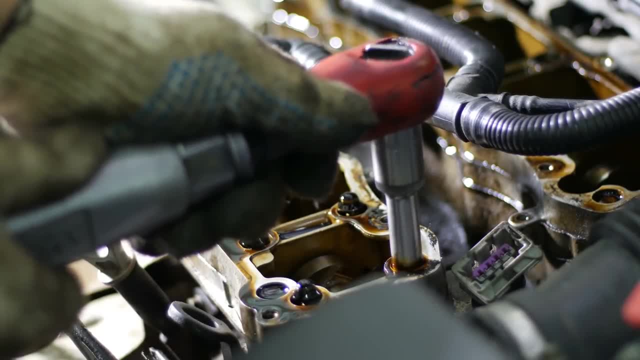 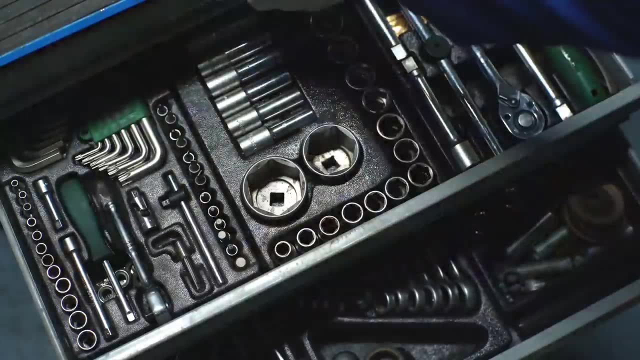 Say you were tasked with building just one car. Say you were tasked with building just one car. If push came to shove you could probably do it, But most of you watching would need to go to school to learn how to put a car together, and you would also need to buy a whole lot of equipment to actually manufacture that. 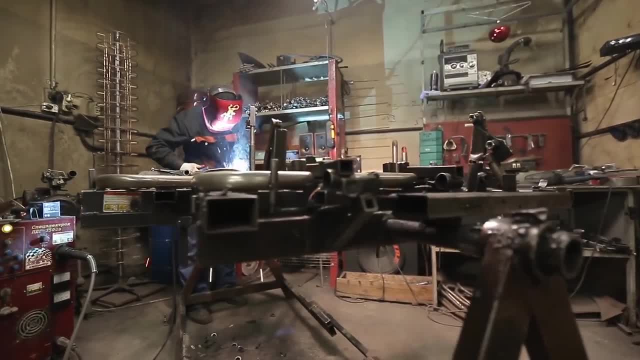 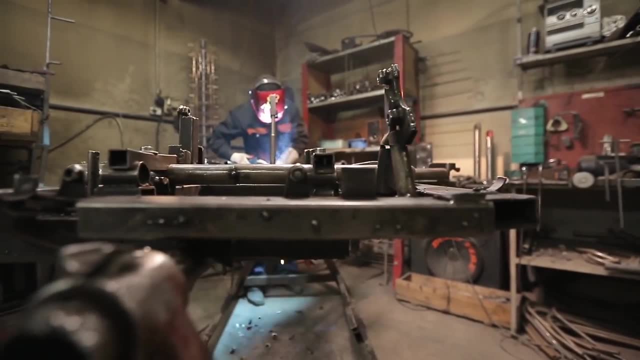 car, This education and a workshop full of tools would cost hundreds of thousands of dollars and take years of your time to put together. If you were to turn around and sell that car at a price that was commensurate with your outlay and effort, that would be an astronomically expensive vehicle, easily hundreds of thousands. 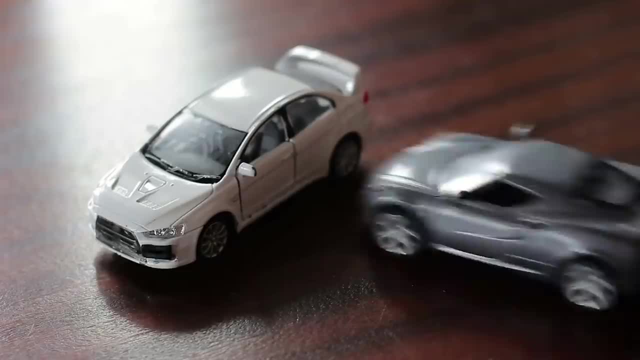 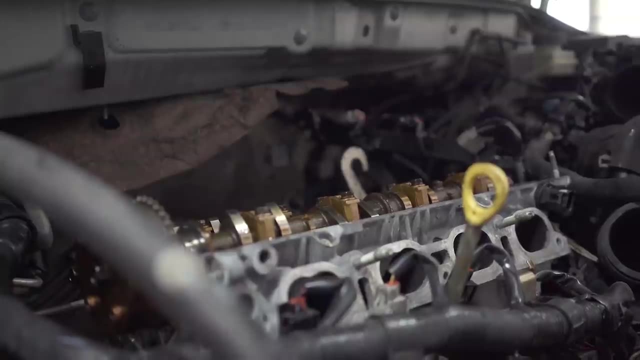 of dollars. But What if you were tasked with building two cars? Well, you wouldn't need to go back to school to learn to build another car, and you could just use the same tools all over again. In this example, the tools and education are the fixed costs. 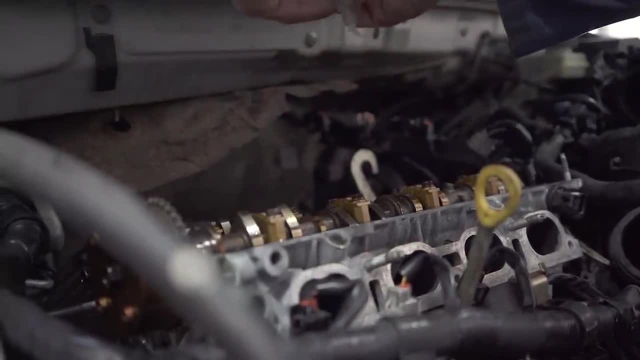 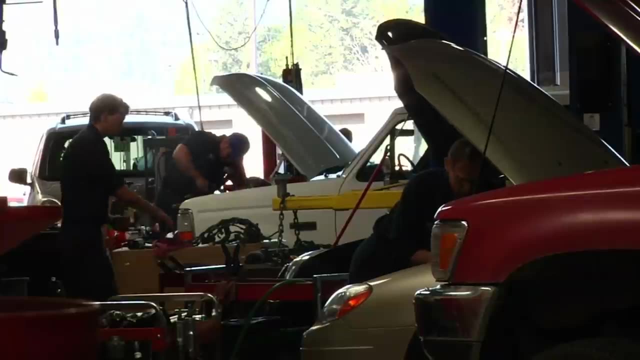 no matter how many cars are made. you don't need to spend anymore on these. As more and more cars are produced, they reflect a smaller and smaller fraction of the total cost involved in making that car. The next big step is scale. Hand tools in a garage workshop are great. 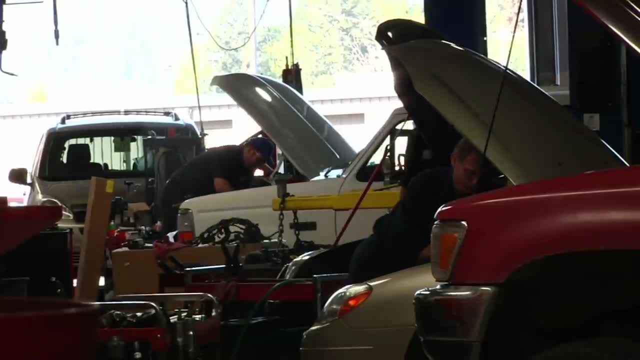 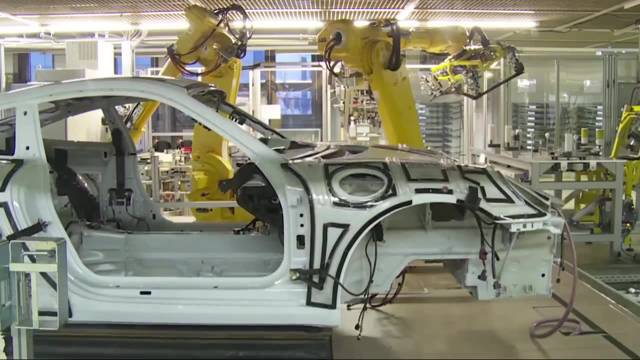 shop are great, but even with the most skilled mechanic in the world, it is going to struggle to put a car together from scratch in less than a month. A full on assembly line on the other hand- well, that's a different beast. Now tasks. 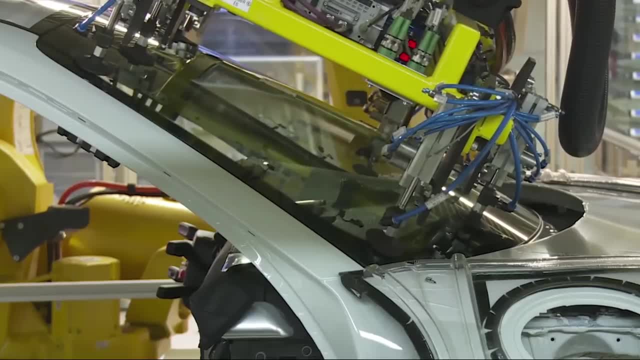 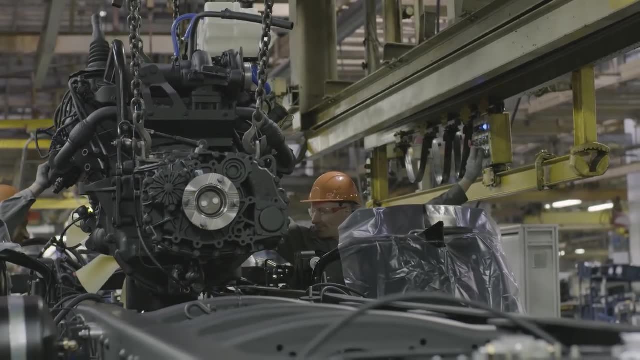 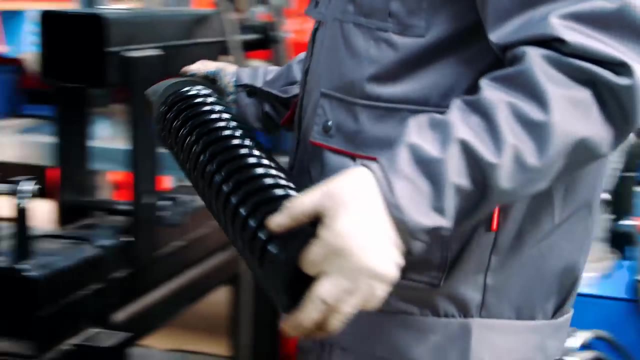 can be broken down into very easy, very repetitive actions that might not require an education at all. What's more is, if they do exactly the same thing day in and day out, you get very, very good at it, inherently making production much more efficient. Basically, if you are ordering a single piece of every component that goes into a car, you will be paying retail price for those parts, but if you are ordering hundreds of thousands of components at a time or, even better yet, manufacturing them in house, you are going to pay much less for them. This lowers the variable costs of production. So all in all, it's looking like a pretty big win for the economies of scale It mitigates. 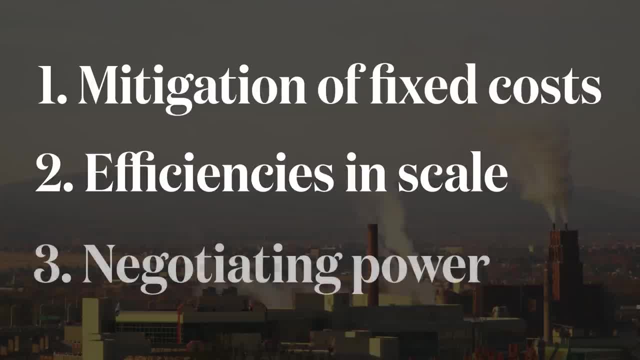 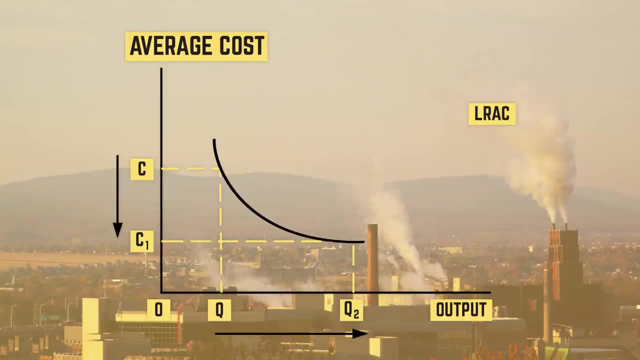 fixed costs, increases output and reduces variable costs. What's not to love? It's pretty easy to graph out this process And see that cost competitiveness will naturally favor those who produce the most. So sure, maybe teslas are a bit too expensive for most consumers today, but as we saw earlier, 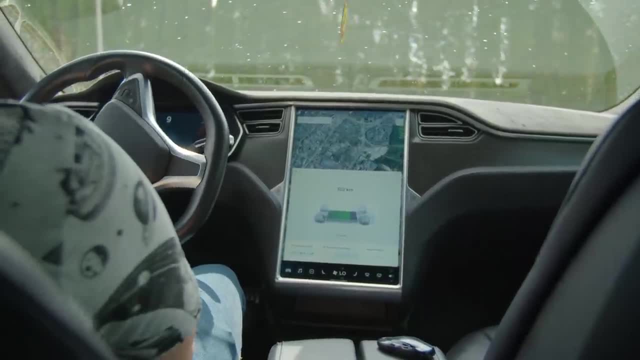 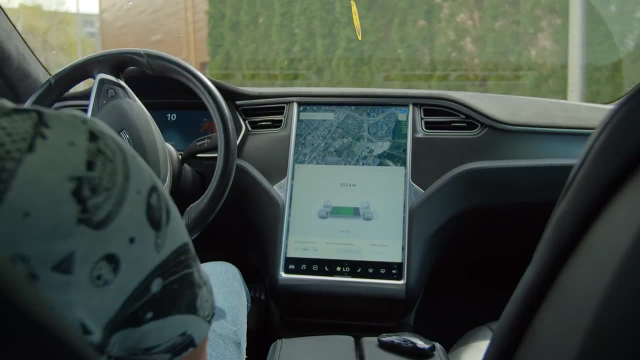 they only make 1 thirtieth the number of cars that toyota does. As soon as they expand into making a few million cars a year, they will have the magic economies of scale on their side and be super profitable, right? Well, maybe, but probably not. 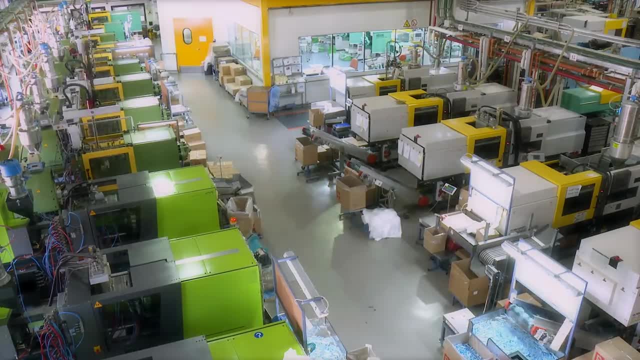 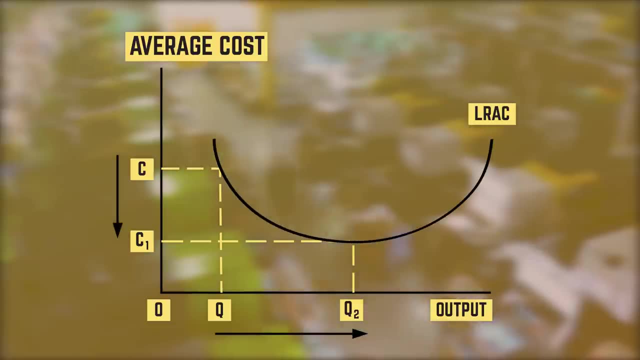 As fantastic as the economies of scale effect looks, it has a dark side. You see, this chart here is not actually complete. It is supposed to look more like this In typical manufacturing: after a certain point, producing more goods starts to cost more and more. This is caused by a reverse of the reasons. we saw all the components getting cheaper. 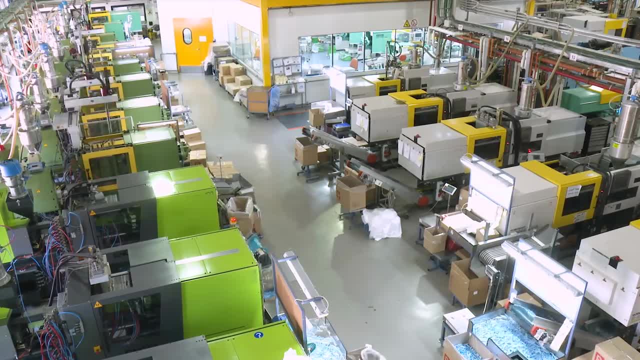 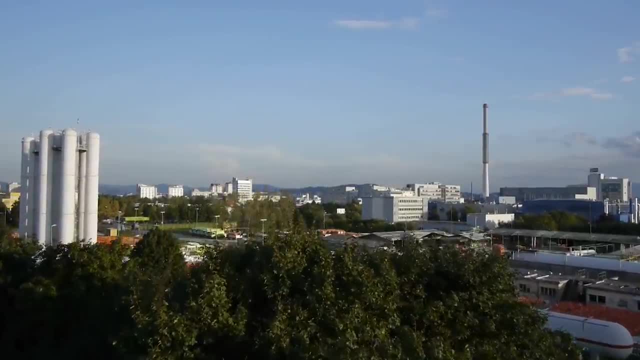 in the first place, Those fixed costs for starters. Either a would be manufacturer is going to have to try and squeeze more and more out of their existing factory or workshop or whatever, Or they are going to need to open up a second location to keep manufacturing. 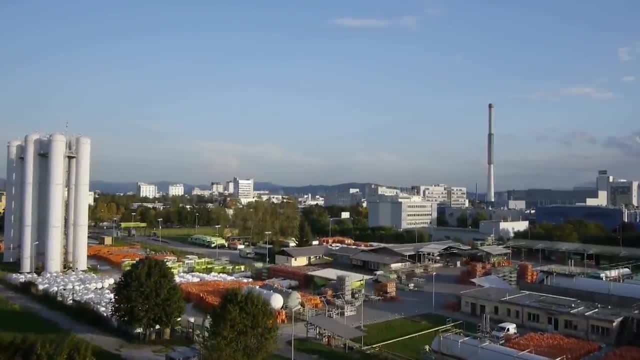 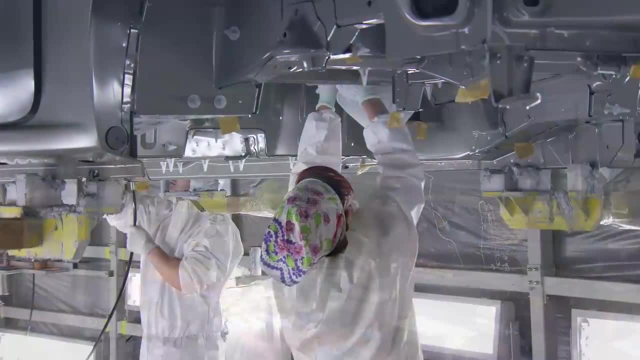 And that's why this chart here is not actually complete. It is supposed to look more like making more cars. This is a huge jump in fixed costs that will need to be shared amongst the costs associated with each individual car. after that, The same thing happens with breaking down processes into smaller and smaller tasks. 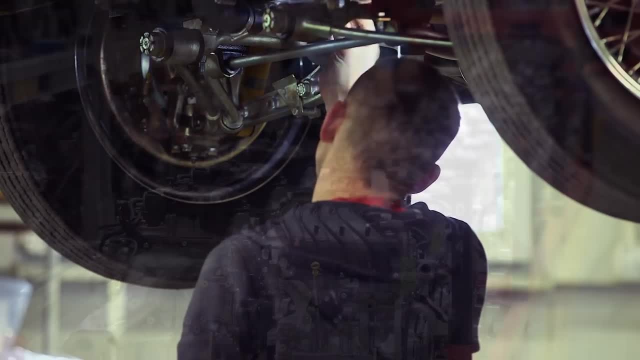 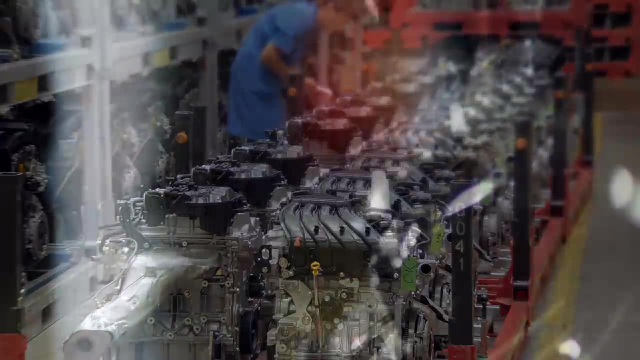 One man. building an entire car by hand is not very efficient. A team working on set steps is efficient, but a huge team of thousands of people, each responsible for one single screw or weld, is just as inefficient as having one person doing the whole thing Eventually. 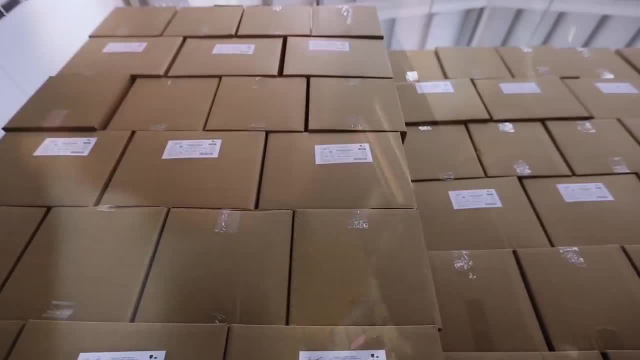 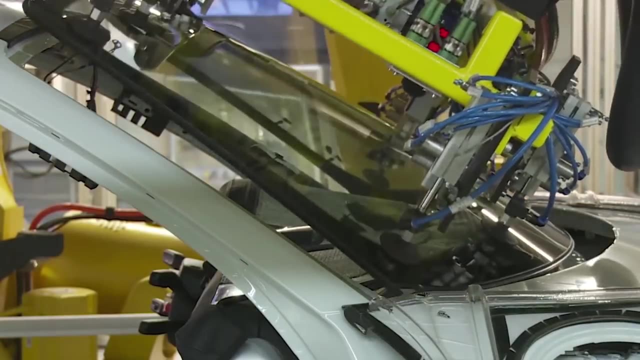 people will just get in each other's way And finally that bulk discount turns into clearing out entire markets. If you want to buy 10,000 glass windows, you get a bulk discount. If you want to buy 10 million, you force demand. 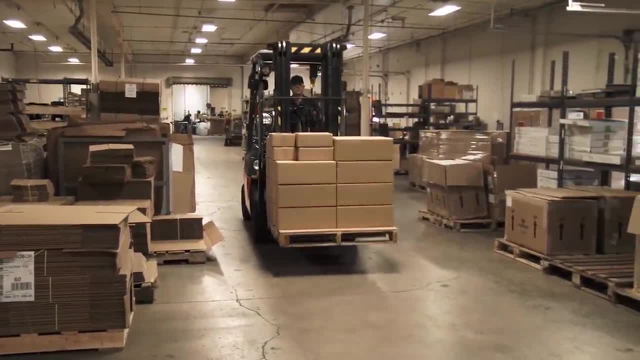 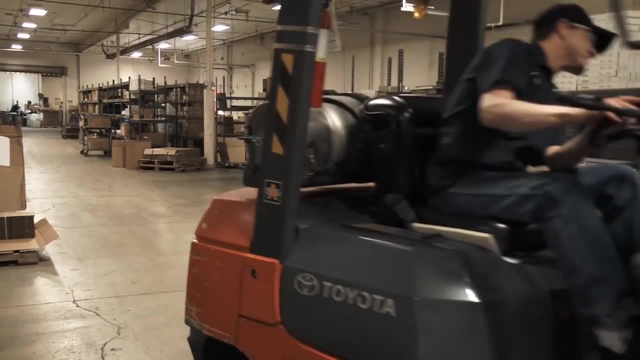 up so high that prices will naturally increase. Call it a personal vendetta of mine, but the loose way that people throw around the idea of economies of scale being the secret ingredient to every business is potentially harmful. in choosing good prices. It's not just a matter of how much you spend, It's a matter of how. 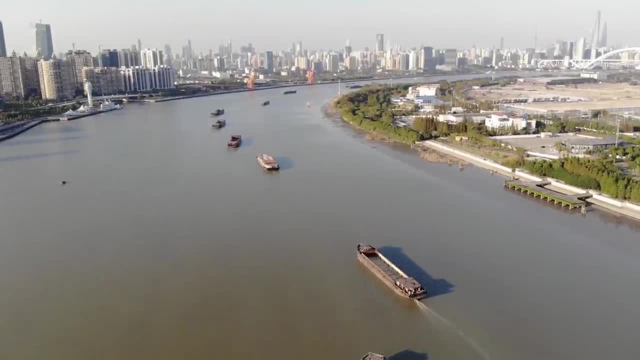 much money you invest, And it's not just a matter of how much money you invest. It's a matter of how much money you invest, And it's not just a matter of how much money you invest. It's a matter of how much money. 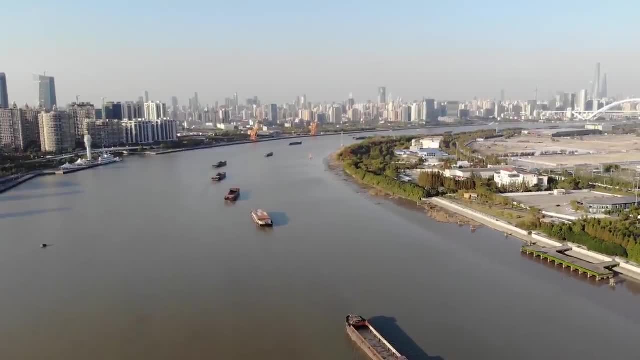 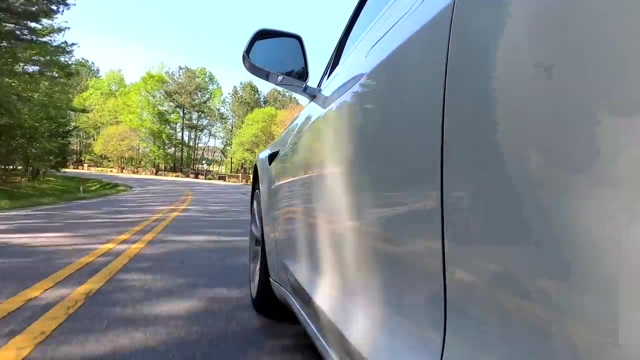 you invest. This should probably be the key takeaway of the video, but nobody will click on a video called the negative marginal cost minimization in high output production. So you know, haha, I tricked you into learning, But maybe we have been a bit too cynical here and missed the point of Tesla entirely Most. 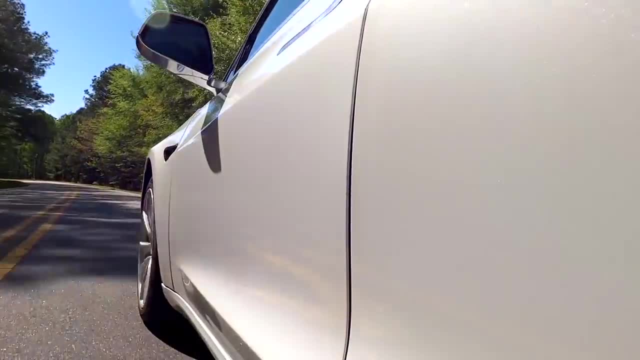 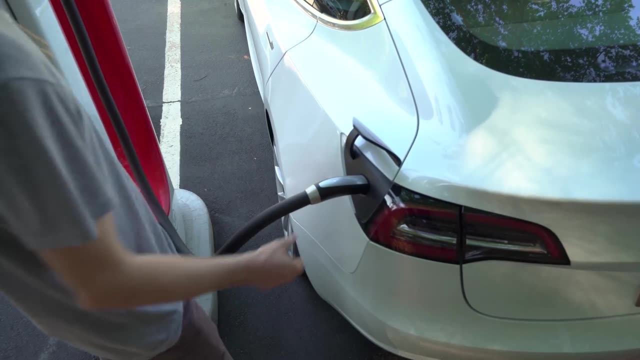 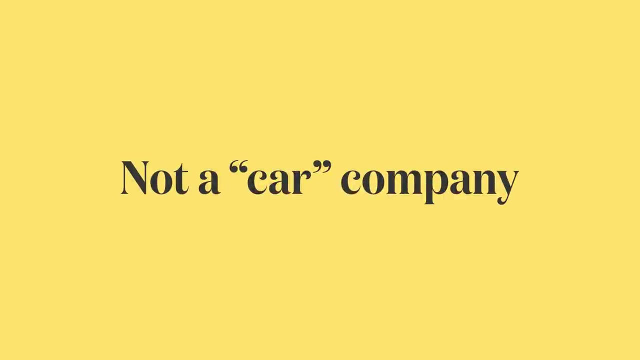 institutional investors agree that a $400 billion valuation for a car company, even one with all of its vertical integration, is absolutely ludicrous, Especially considering all of the factors we have already explored. But maybe Tesla is not a car company at all. I mean sure it builds cars, but not many. 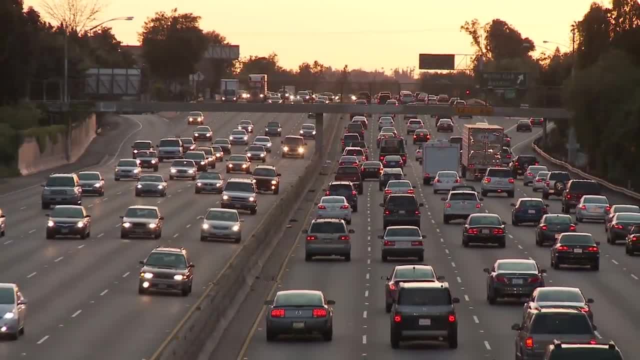 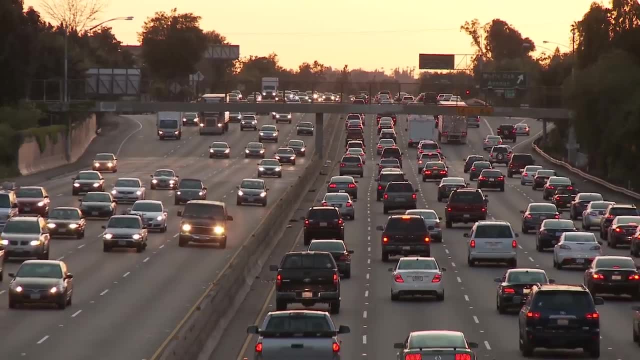 of them, and they are really only a means to an end of efficiently getting people from place to place. What is much more exciting, especially to investors, is the final step of the company's plan to control everything related to road based transport. the idea 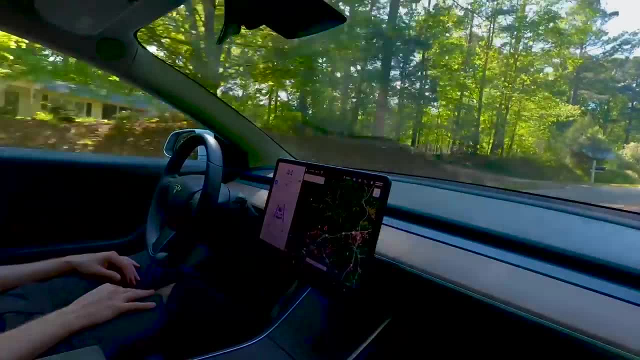 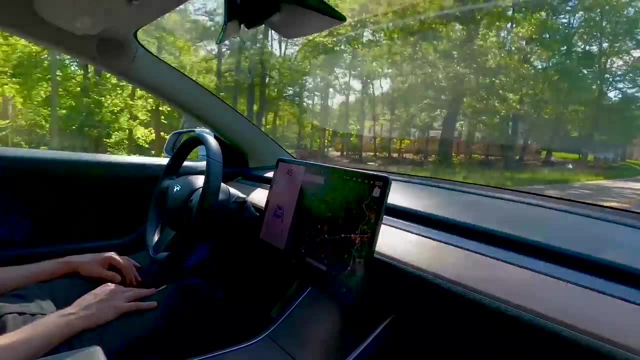 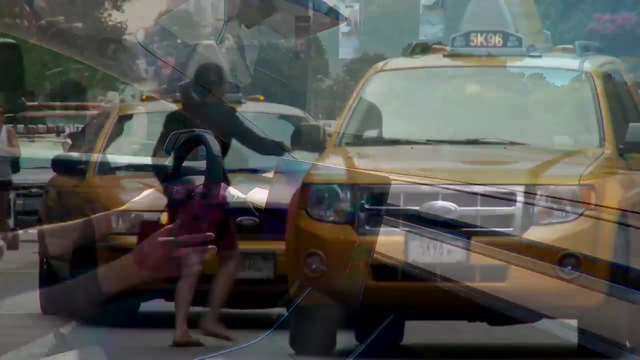 of car ownership itself. Tesla is quite famously developing systems for self-driving cars. right now, these systems are little more than a cool party trick, but they have some much more serious long term potentials. It could become their very own transport network. Taxi companies and uber drivers make money by purchasing vehicles and using them to transport passengers. 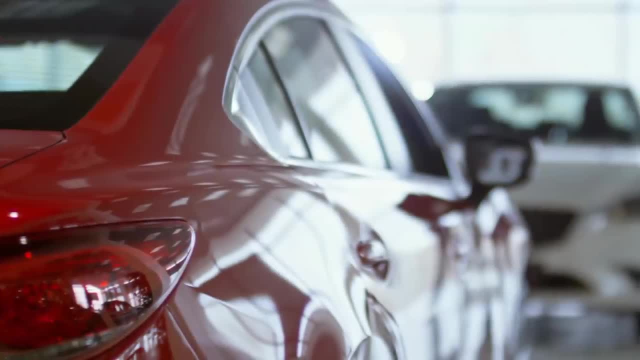 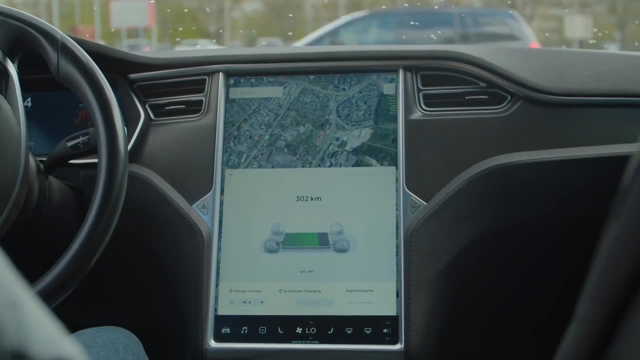 which means there is more money to be made in moving people about than in simply selling a car as a one time transaction. Even a range topping Tesla Model X sells for under $100,000 in the US today, Which is obviously a lot of money. but that same car, if let loose to act as its very 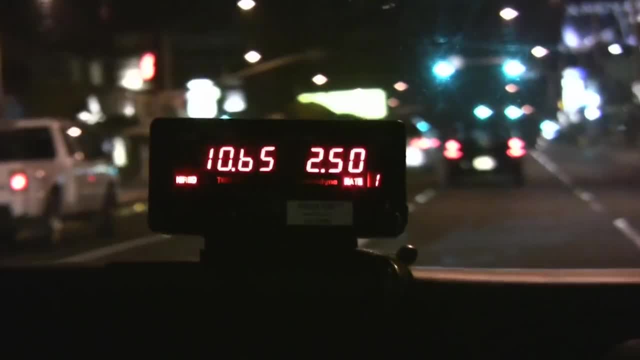 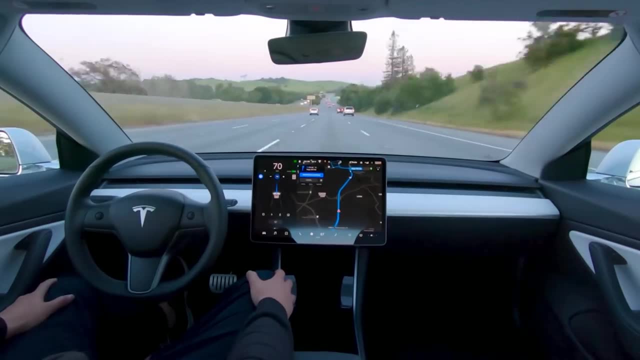 own uber driver could make hundreds of thousands of dollars before eventually being retired. Elon Musk has already spoken quite freely about a future where nobody owns a car, which would be very unusual rhetoric for a car company CEO, had it not been for this more holistic. 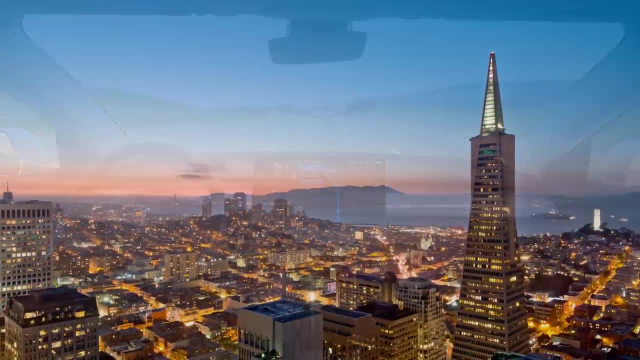 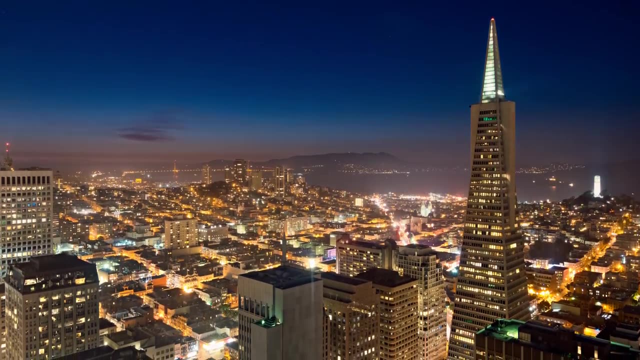 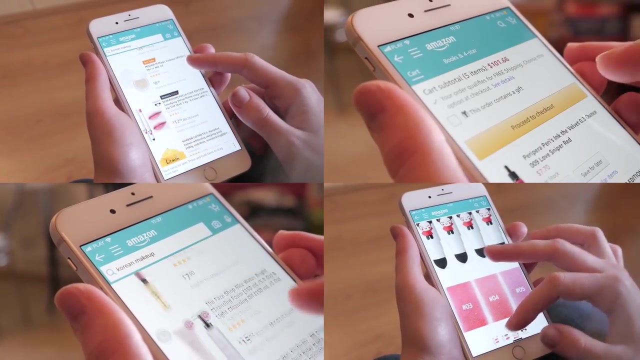 approach to a transport solution. Now, what investors hope this means is that Tesla is more of a tech company that just so happens to make cars, Rather than a car company that just has some cool tech. Technology has the advantage of being able to achieve the aforementioned economies of scale far more efficiently than other types. of businesses like retail oil and gas, health care, pharmaceuticals and, yes, of course, even auto manufacturing. That's why, today, 7 of the top 10 most valuable companies in the world are tech companies. So the cynical analysts are right: Tesla, the car manufacturer, is not worth even a.